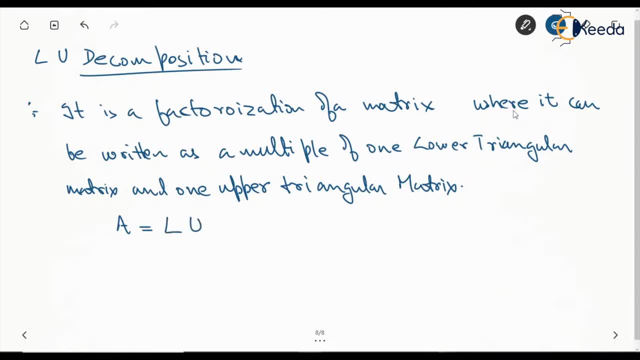 Obviously, this is going to be a square matrix, Right? So let's see how we are going to do this. Let's say we have for A being a three cross, three matrix. what we can do is, of course, we can take all this. 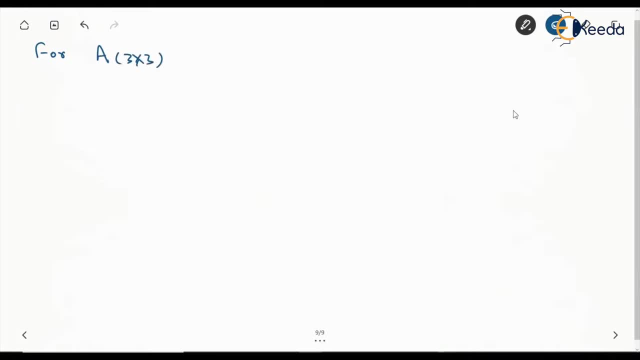 a one, one, a two, two, all this three cross three elements. like nine elements will be there. So what we are going to do is we are going to take all this. nine elements will be there. So what we can do is for this. 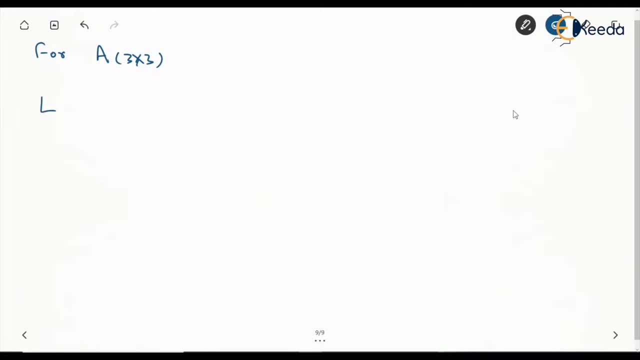 a equal to three cross three matrix. we can have this l as its diagonal elements being one. of course, upper elements will be zero and rest are the unknown. So l two, one l three, one l three, two. These are the unknowns and for this we will have 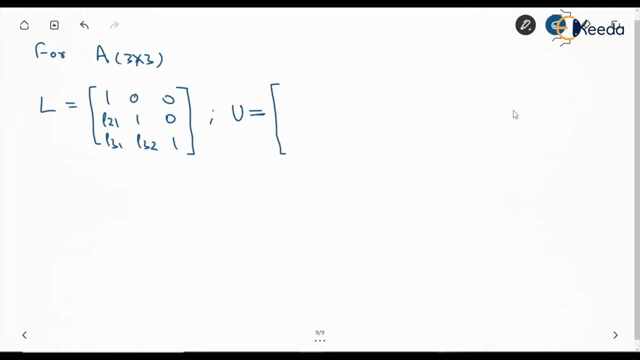 as with all the unknowns other than zero elements, so it will be u one one, one, two, one, three, zero, two, two, two, three, zero, zero. and u three, three. or else we can also present it as l being l one one, zero, zero, l two one. 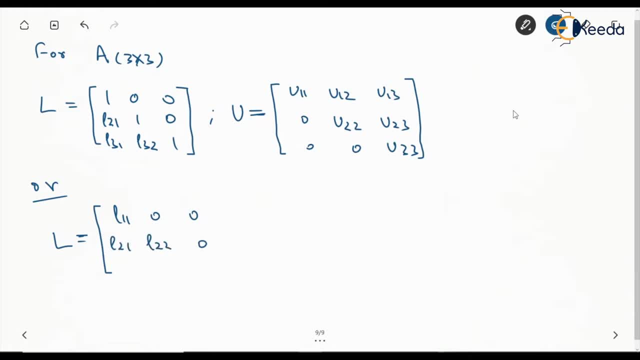 l two, two, zero, three, one, three, two, three, three, with u equal to one, u one, one, u one, two, zero. again. this lets say these are going to be one, these are going to be one, these are going to be zero u three. so in one of it we are going to make 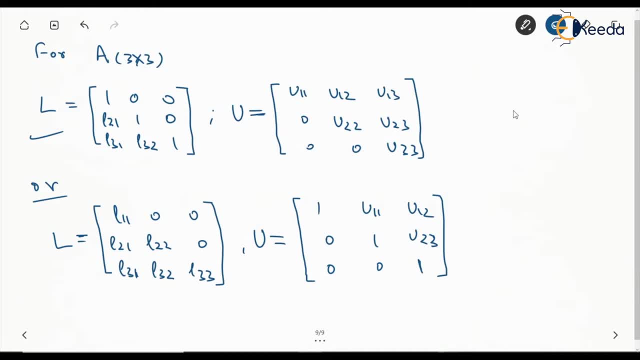 the diagonal elements to be one and other to be unknown. of course this is upper triangular, so lower elements are zero and in another one we are going to for like for l is going to be upper triangular elements to be zero and all other to be unknowns. as, in terms of l, 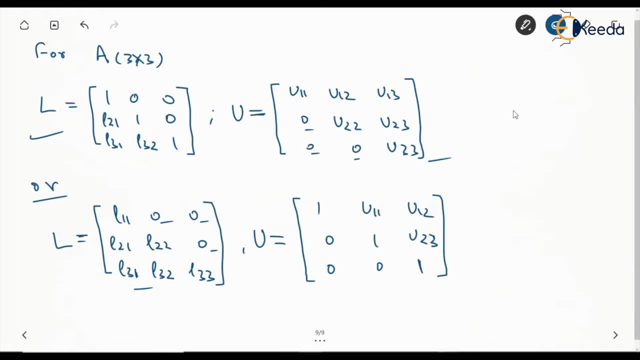 whereas for upper triangular matrix we are doing lower off diagonal elements to be zero, diagonal elements to be one, and these are the unknowns. so these are. this is two methods: either you make l diagonal elements to be one or u diagonal elements to be one, like that. 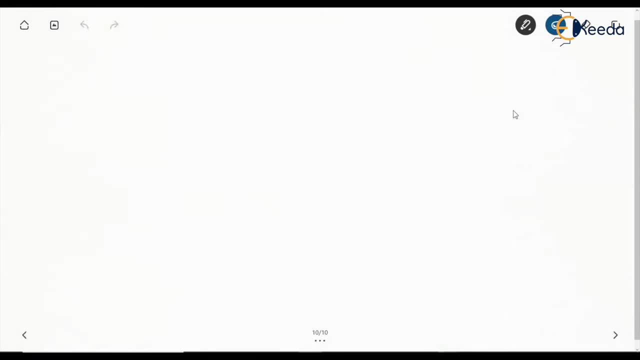 so lets see how we are actually going to get the solution for this. so far, we know that for a system of linear equations we had, we had we had- ax is equal to b. this is what we know now. if a is written as l into u, this becomes: 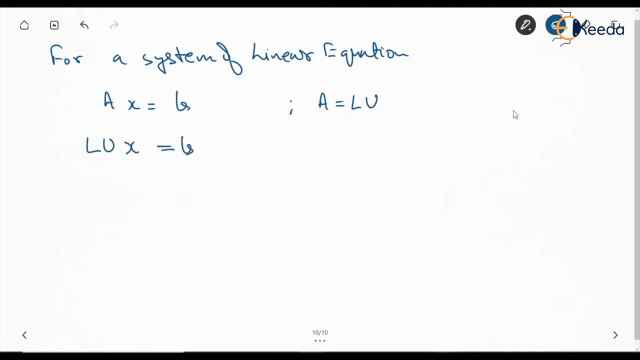 l u x, equal to b. what if we write u into x is equal to y. in that case, this becomes l into y, equal to b. now, from here we can find y because it is going to be triangular. l is going to be triangular, so it will be easy to find y. 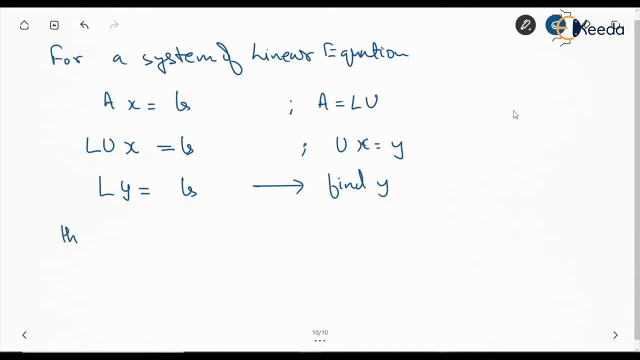 and then we can substitute in the relation u, x is equal to y, to find x, we can find x, and thats it. we will get the solution right. so lets see one case. so lets say we have compute l? u, factorization of the matrix. so this a. 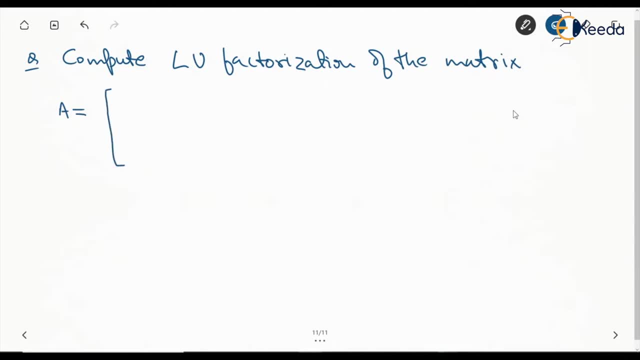 is given by two, one, one, four, five, two, two minus two, one zero. lets say we are writing it in the form of l? u, as: lets say it is: one zero, zero, l two. one zero, zero, l three, one, l three, two, zero. lets keep this. diagonal elements one. 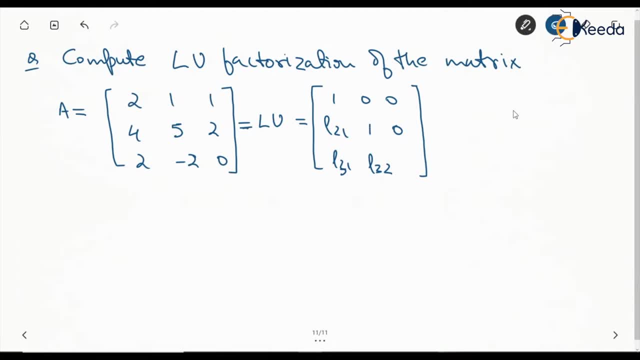 in this form, one and one. then we will have all the elements to be unknown in: u: u one one, u one two, u one, three. obviously these elements are going to be zero. so u two, two, u two, three and u three, three, right. so if we multiply l with u, 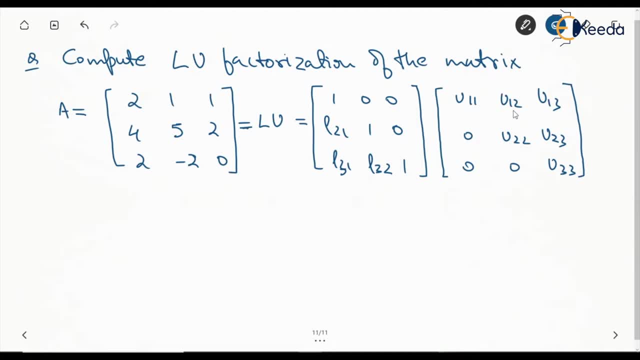 we can compare the elements of a and then we can find the values. so comparing l? u with elements of a. what we are going to do is: lets see first row, first column. so if we multiply this row with this column, we are going to get one into u, one one. 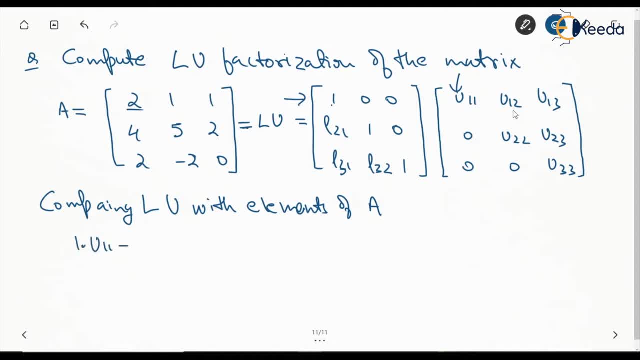 so one into u one. one will be equal to this two, so we can directly write u one. one is going to be two. then we will move to the next element, one. so this is going to be first row and first column right, first row of l and first. 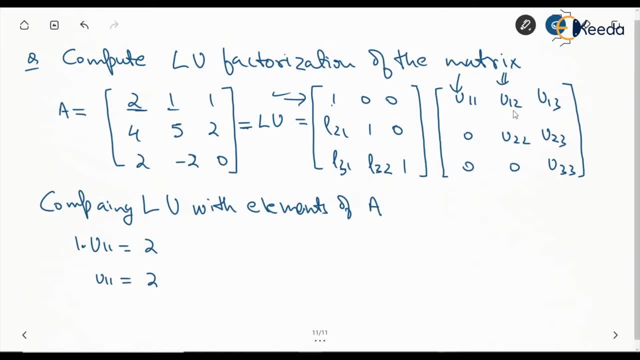 column of u. so this is going to be a one two is equal to one. into u one two and that that's it. other elements are going to be zero. so we can say: u one two is going to be one because a one two is one third. 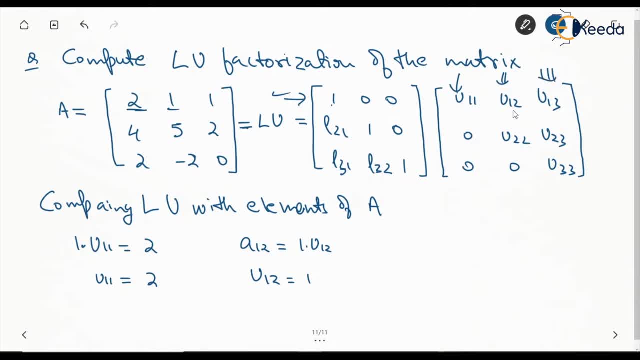 one, so third column of this and first row of l. so as we get this one, so this is going to be a a one three is equal to one- into u one three, so we can write u one three is going to be one, so we have found three elements. 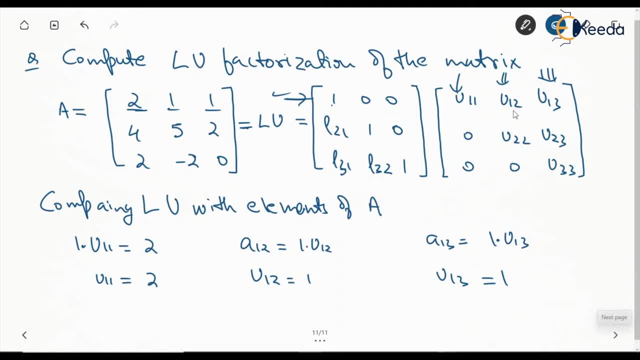 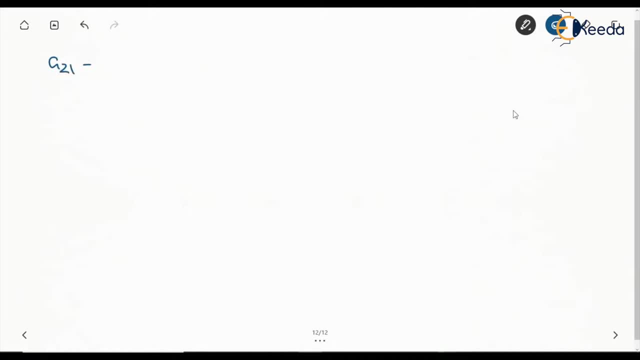 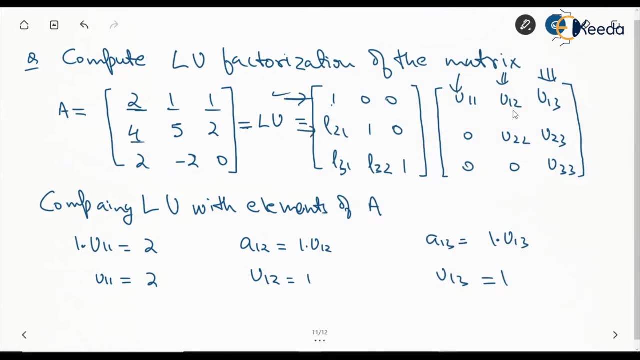 and all three elements are from u. moving to the second row of a, we can see a two. one is going to be a two. one which is four is going to be the product of second row, with the first column right then five is going to be product of second row. 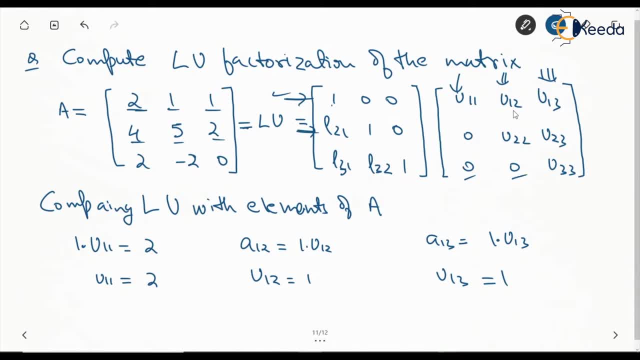 with the second column, then two is going to be second row with the third column, and likewise, two is going to be third row, first column. third row, second column, third row, third column. likewise, we are going to compare all the elements so that we can get the unknowns. 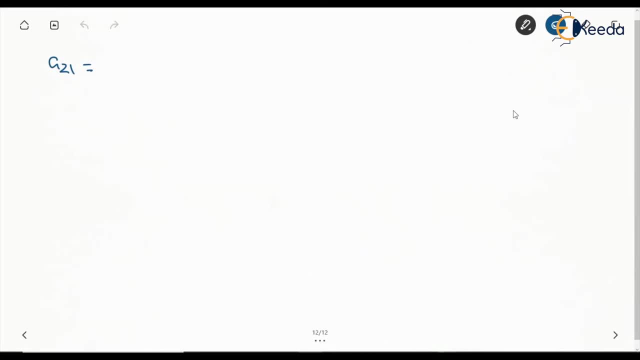 so let's proceed. this a two one is going to be a l two one into u one one, and now that u one one is already known, which is two, we will get l two one is equal to. since a two one is going to be four, this is going to be two. 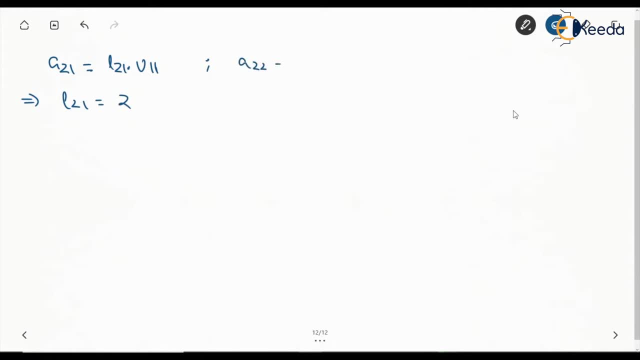 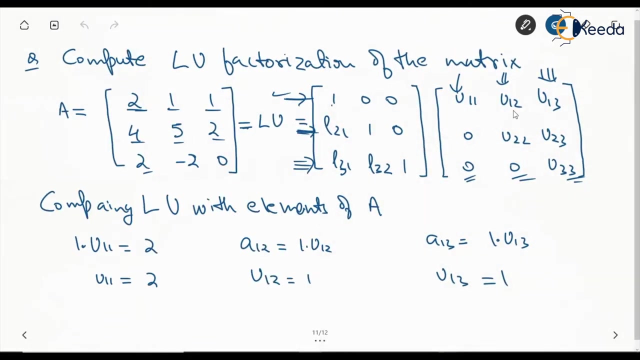 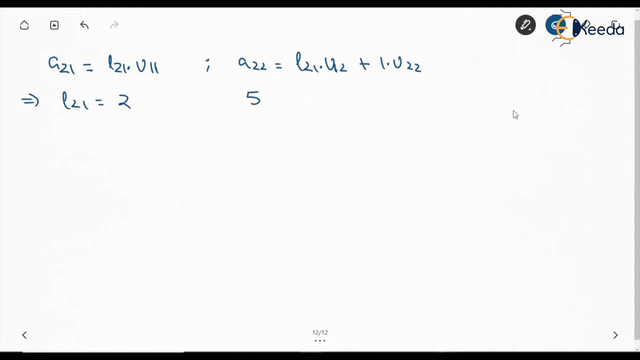 next is a two. two is going to be l two. one into u one two plus one into u two two. a two two is five and we have already found some of the values, so this is going to be five. so this is five equal to two into. 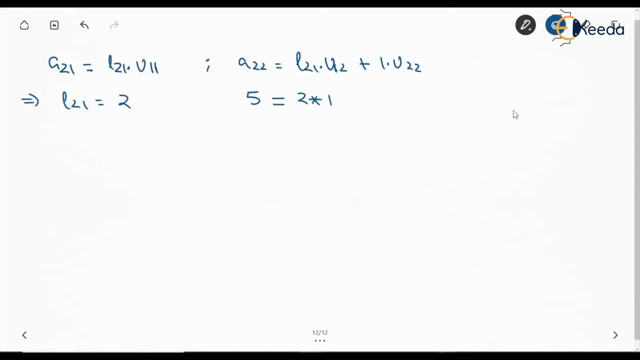 one. now that l two one is known u one two is also known plus u two two. so from here we can find: u two two is equal to three. moving to a two three, a two three will be l two one into u one three plus u two three. 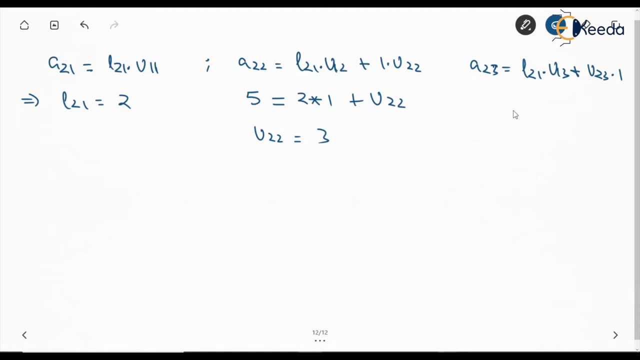 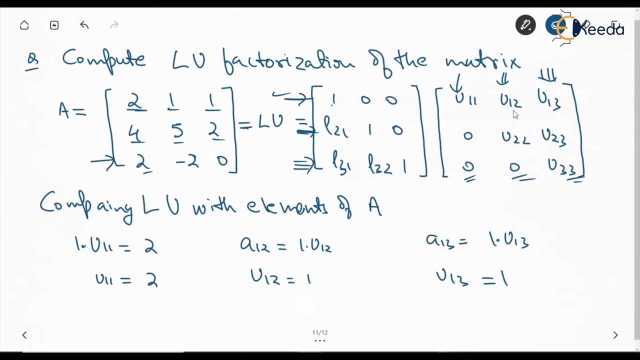 into one, so this is going to be two equal to two into one, plus u two three and u two three becomes zero. so one more row is done. now we can move to third row of a, and we will find this by multiplying third row of l with 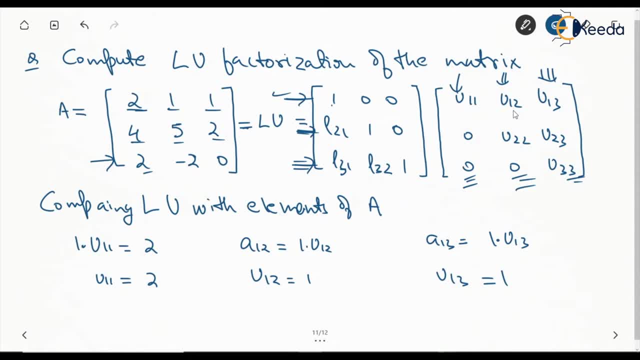 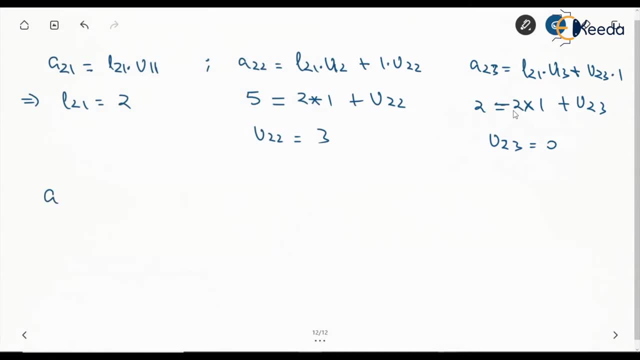 first column of u, second column of u and third column of u, like that. so this is going to be a three one is equal to l three one into u one one. u one one is already known, so a three one is two, so l three one becomes. 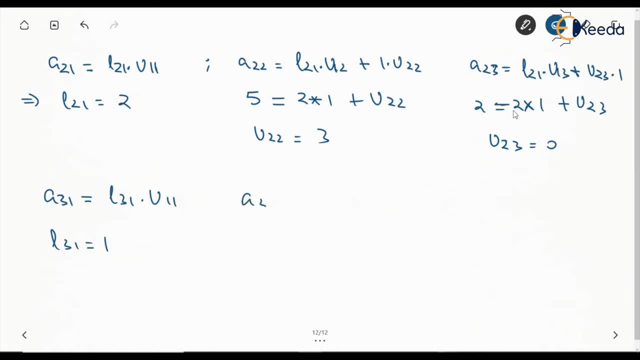 one. next is a three two equal to l three one into u one two plus l three two into u two two. putting all the values we have already found, like l three one is also found now. a three two is minus two. so minus two is equal to. 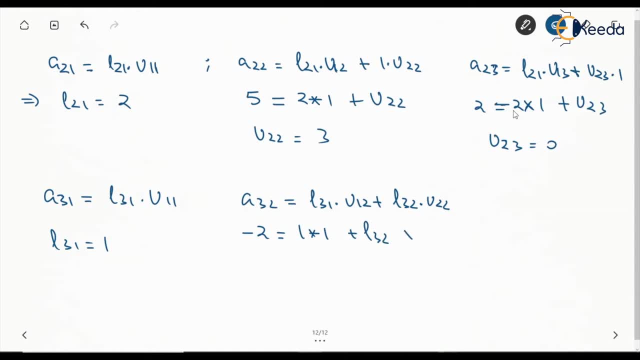 one into one plus l three, two into three, and this gives l three two equal to minus one. the last element is a three, three, which is going to be l three. one into u one, three plus l three, two into u two, three plus directly u three, three. 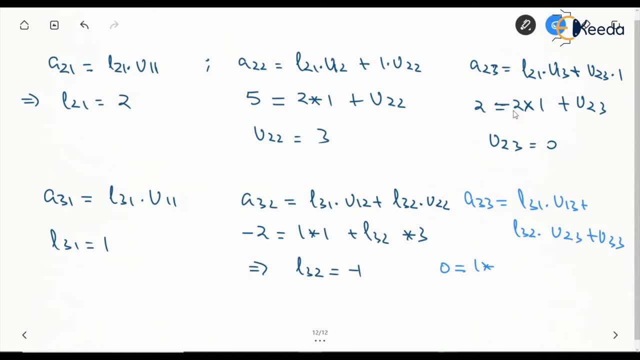 this makes it zero, equal to one into one plus minus one into zero, plus u three, three, and we get u three. three is equal to minus one. so we have found all the elements we can arrange it and we will get it to be as a equal to l? u. 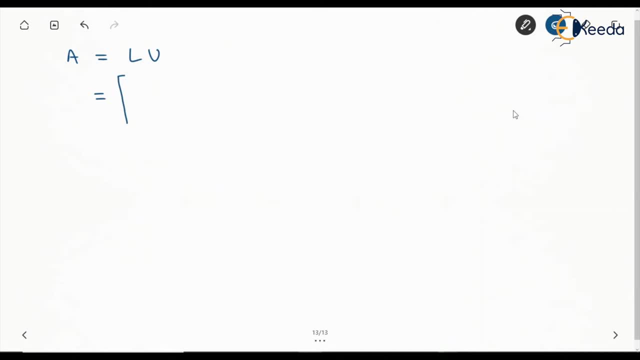 will be one zero zero, two, one zero, one minus one one, and u will be two, one, one zero, three zero, zero, zero minus one. now lets see if we had, for a, x is equal to b, we have a, x is equal to b. and we have what if? 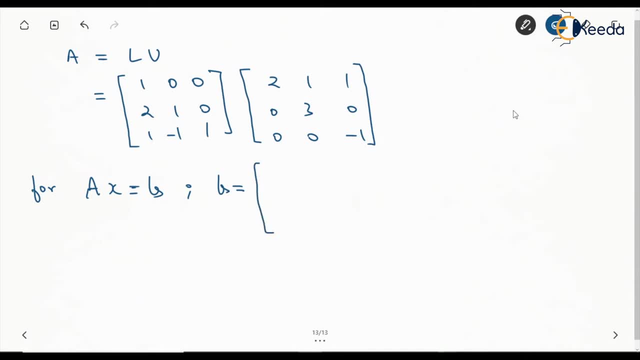 this b was one, two, two. lets say it was one, two, two, right, and we have to solve for x. so the first thing is, instead of a, x is equal to b, we can write l into y equal to b, because we are taking y is equal to. 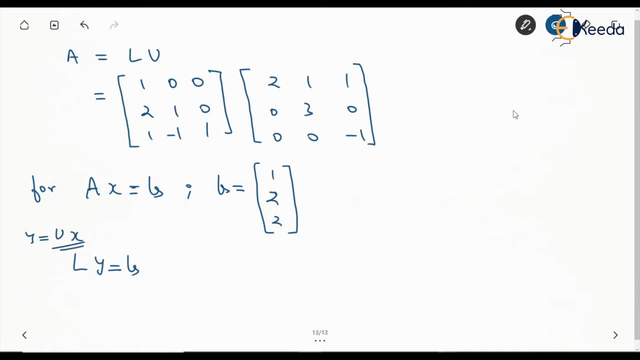 u into x, right, so this is going to be one zero, zero two, one zero one minus one, one into. lets say these elements are for y. we have, lets say, y one, y two and y three. so this should give you b, which is one, two and two. 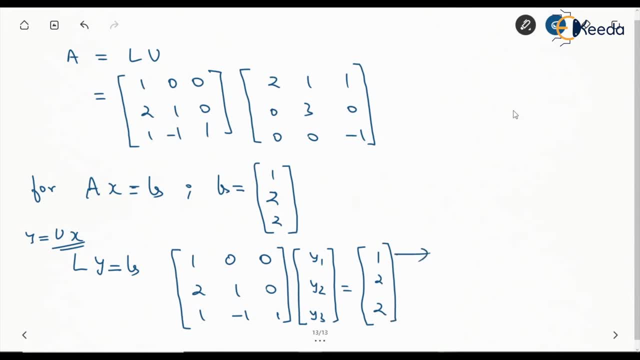 so from here we can start solving the first equation, then second equation, and then third equation. so if we are solving the first equation, we can see one times of y one will give you one right, so this y one is going to be one. then we can substitute. 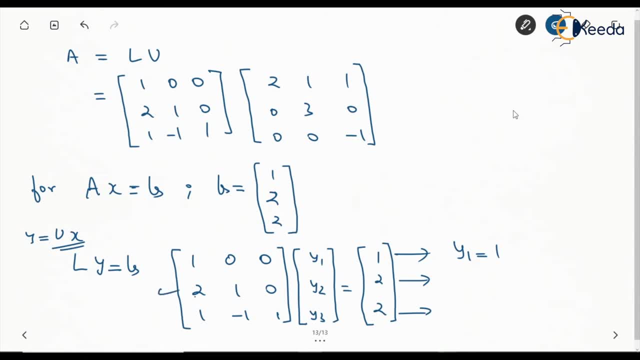 y one for the second equation. so this is two times of y one plus y, two plus zero equal to two right. so in that case we can see that y two is going to be zero, right. we are substituting right. we have already done in the gauss elimination. 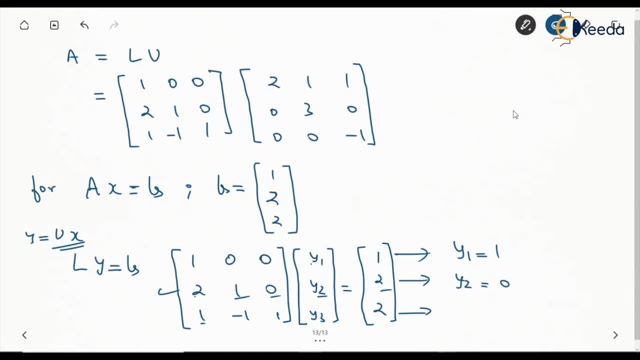 and the third one is y. one is known to be one, y two is zero. so plus y, three is equal to two and this gives y three is equal to one right. so we have found y. y is one zero one. now we can move for u. x is equal to. 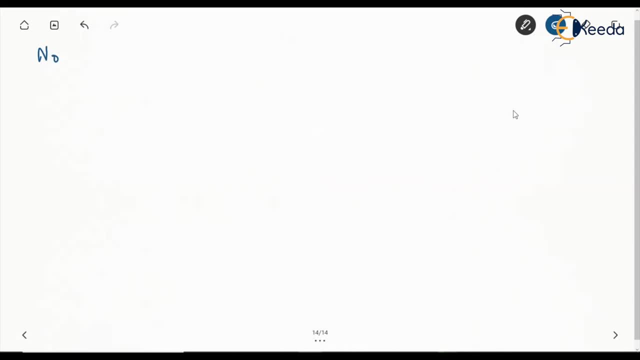 y. now u, x is equal to y, so u is two one, one zero, three, zero, zero, zero minus one. and let's say x is x one, x, two x three, where we have also found y, y is one zero one. so what we can do is we can start with the third equation. 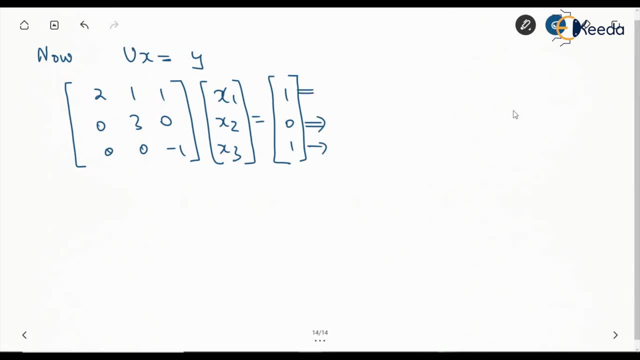 then move to second equation and then move to first equation. right, so from first equation we can directly see: minus one times of x three is equal to one. so this will give: x three is equal to minus one now substituting this, so zero times of x one.